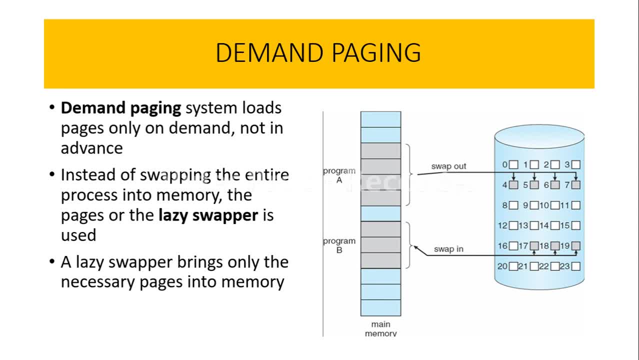 hello everybody. in this video we are going to discuss about the demand paging. so this demand paging is a common technique, what we can use to implement the virtual memory. so what exactly you mean by this demand paging? so let me tell you: demand paging is a technique or system which is going to load only the 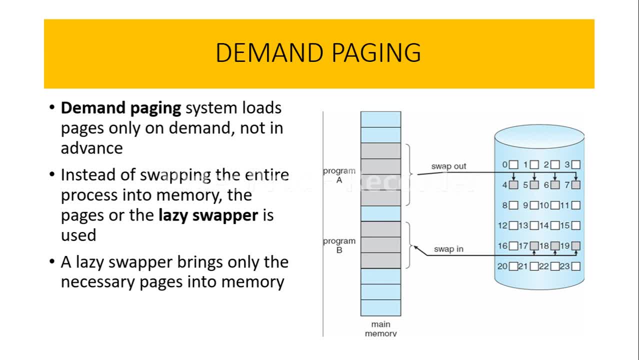 pages on demand. that means it is not going to load the entire program on to the main memory for processing, but it is going to load only those pages which are required for processing purpose. okay, so, as we know that the process is normally residing on the disk, okay, and whenever we wanted to execute this process, we are 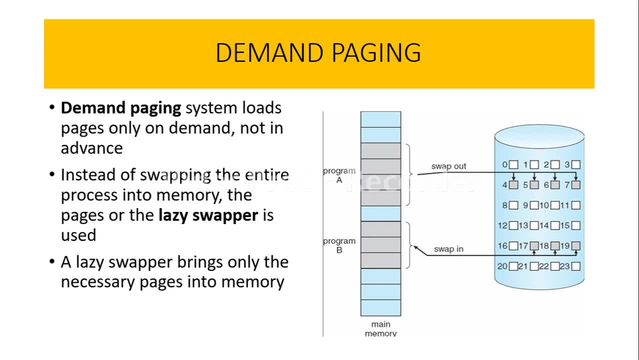 going to swap it into the main memory. now, the task of this demand paging is to load only those pages of the process which are required for processing for the execution purpose, instead of loading the entire program and wasting the memory. okay, so to swap the required pages on to the main memory, we are going. 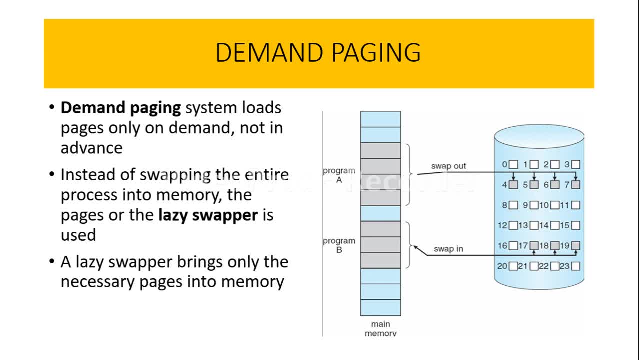 to use the concept of lazy swapper. now, the task of this lazy swapper is to bring only the necessary pages on to the main memory. now, if you see the diagram over here, this is the diagram for showing the transfer of pages from the disk to main memory or vice versa. okay, so, as you can see here, whatever the 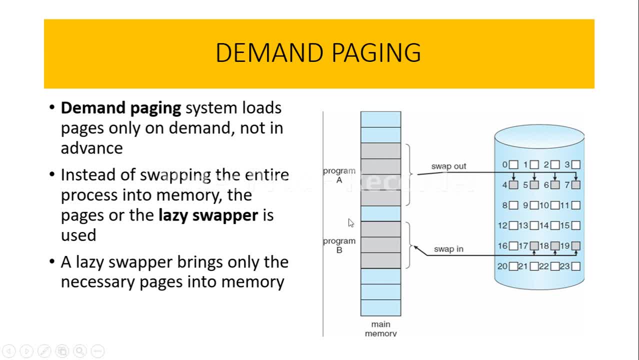 pages are not required by this program a. as you can see, we are having two programs, so the pages which are not required by program a are swapped out. swapping out means we are going to remove it from main memory and we are going to place it back on to the main memory and we are going to place it back on to 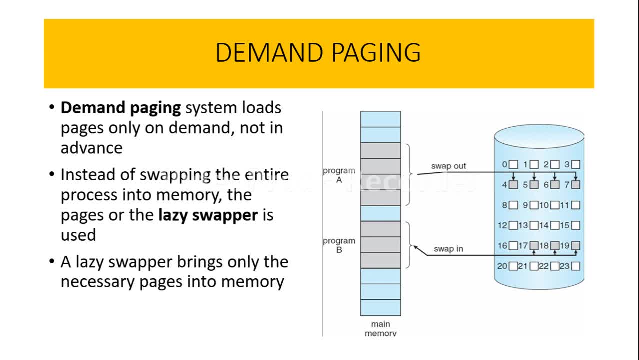 the disk. ok, and similarly you can see here, the pages required by program B are swapped in. okay, so like this, we are going to use the concept of lazy swapper to swap in or swap out the pages which are required or not required by the program into the main memory. okay, so this is the basic concept of demand. 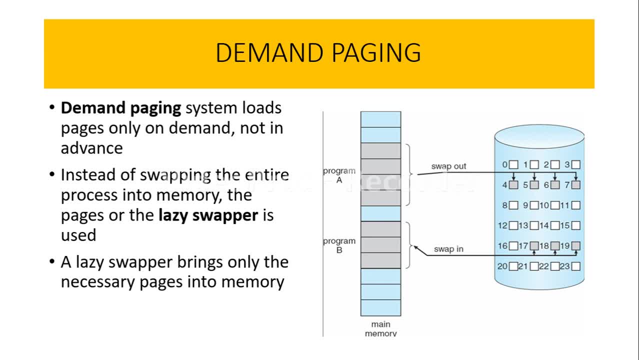 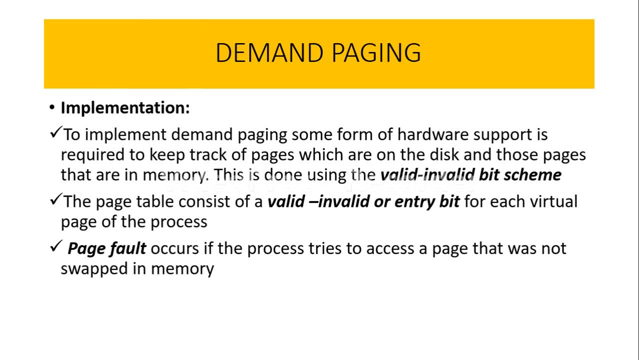 paging. now how exactly we can implement this. if you want to implement the concept of this demand paging, we need a special kind of hardware support. this hardware support is going to keep track of the pages. when we say keeping track of the pages, that means it will keep track that which are the pages. 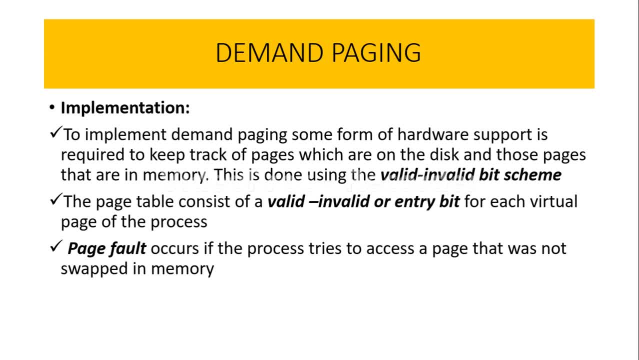 which are placed on the disk and the pages which are there in the main memory. and this tracking of the pages can be done by using a scheme called valid invalid bit scheme. okay, so the we are having actually a page table which is going to have this scheme, that is, valid invalid entry bit scheme. okay, 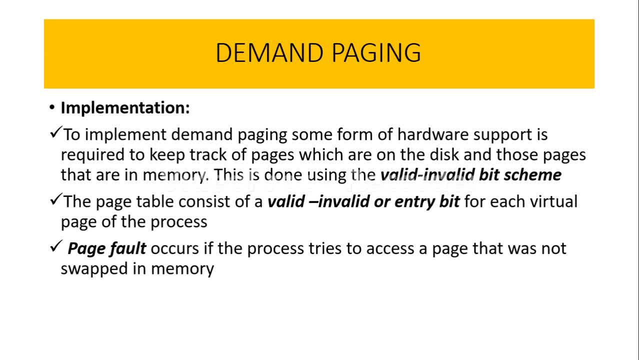 and there is one more point here called page fault. this page faults are occurring particularly when the process is trying to access the page which is not swapped into the main memory. now let you see how to get the page of the page, and then what we are going to do now is we are going to 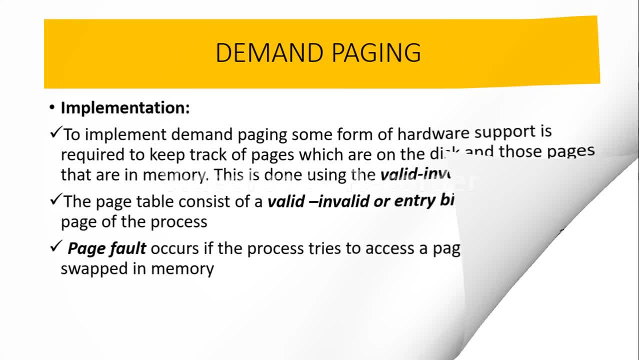 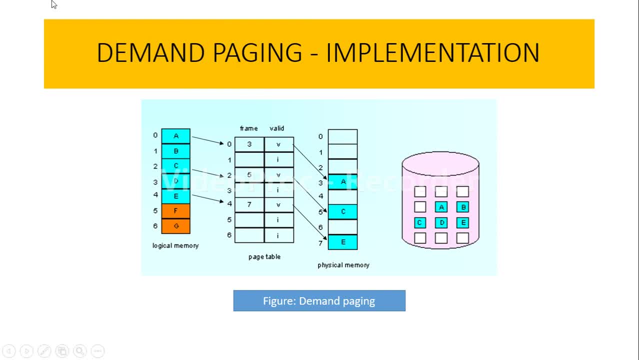 let us have a visual idea about this implementation. So this is the diagram for implementing the demand paging. Now here, as you can see, we are having the logical memory, we are having the physical memory and we are having a page table in which we are going to. 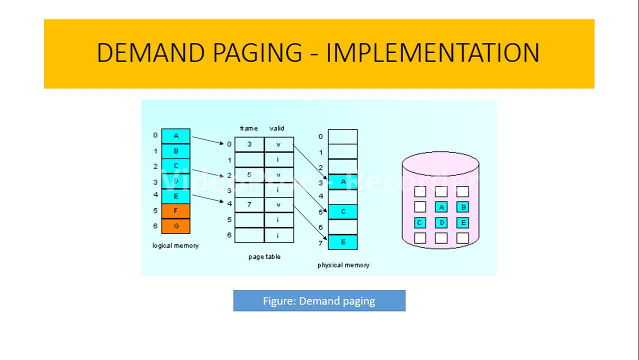 use the concept of valid invalid bit scheme. So, as you can see here, the entry bit for pages which are bought into the physical memory are set to the letter v. v indicates valid. you can see here: and i indicates invalid. Okay, the entry bit of the pages which are not currently on the memory. 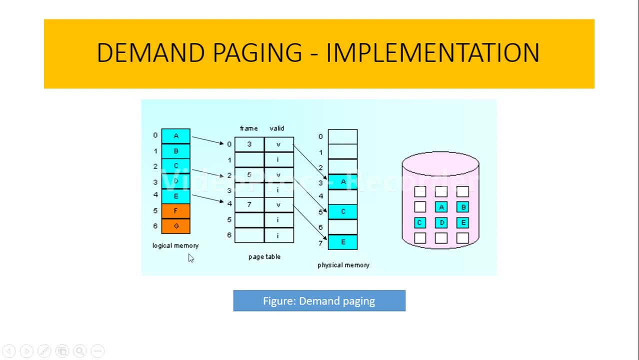 are marked. as i Now see here in the logical memory we are having all these pages containing certain kind of data. Okay, and here you can see in the page table. we are going to keep track of the page Now. you can see there are certain pages where we have written v. v means valid. that means these are: 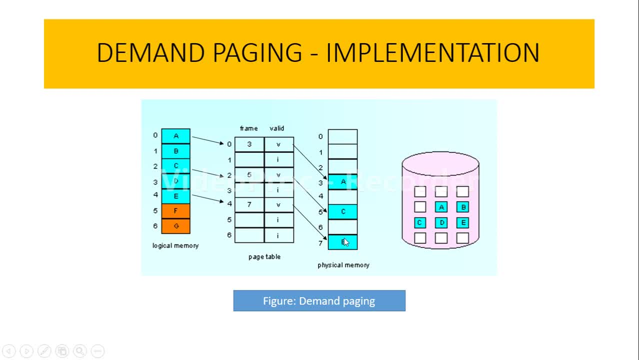 the pages which are loaded onto the physical memory. Okay, so next comes the i- i indicates invalid pages. that means these are the pages which are residing on the disk but they are not on the physical memory. Okay, and whenever the process is getting executed,